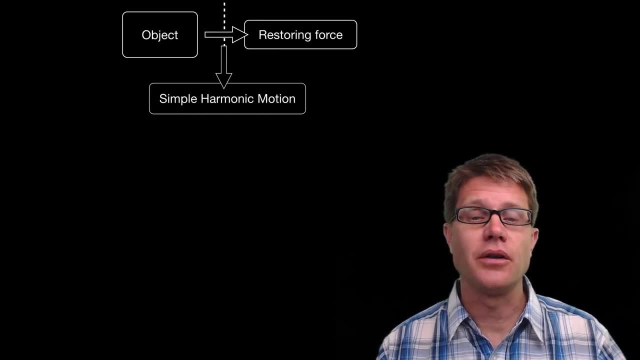 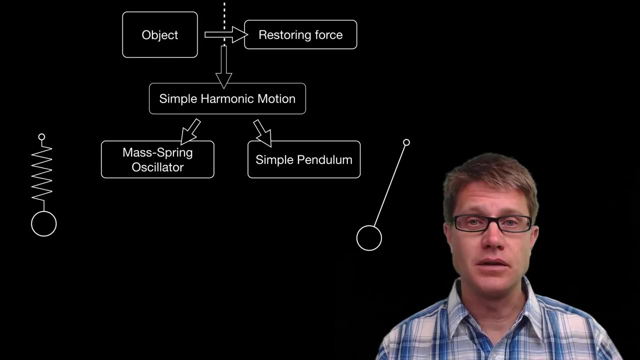 object moving towards equilibrium based on restoring forces. we call that simple, harmonic motion. And so here are the two types we will talk about in AP Physics. And so what we are going to talk about in AP Physics Now, an important characteristic with each of these: 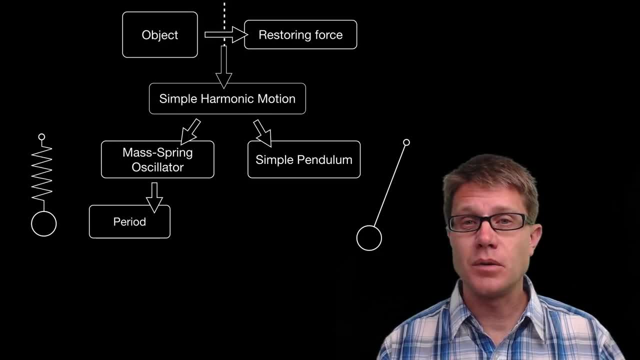 is the period of that harmonic motion Period is always going to be measured in seconds and it is time. So it is the time it takes on this oscillating spring to move from here, to bounce up and then to bounce back again, Or for a pendulum to swing from here over. 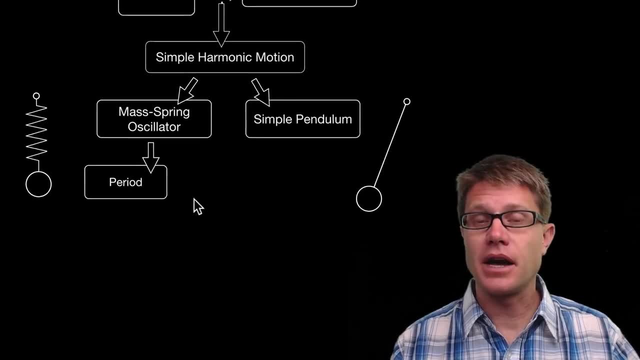 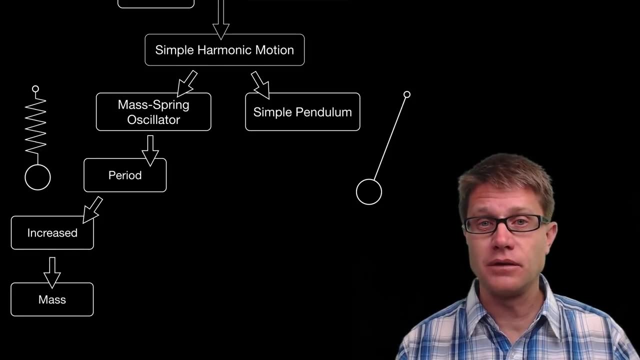 to here and then back again, And so in a mass spring oscillator. how do we increase the period? Well, the easiest way to do that is simply increase the mass. As we increase the mass hanging from the spring, the period is going to get longer, And so what we are going to? 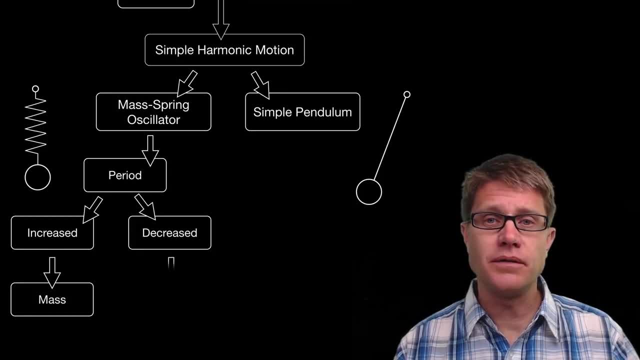 make it longer. How do we decrease it? Well, we can change the stiffness of the spring. As we make it stiffer, then we are going to make that period go down. What about a pendulum? How do we increase the period of a pendulum? Well, we do that by just simply changing the 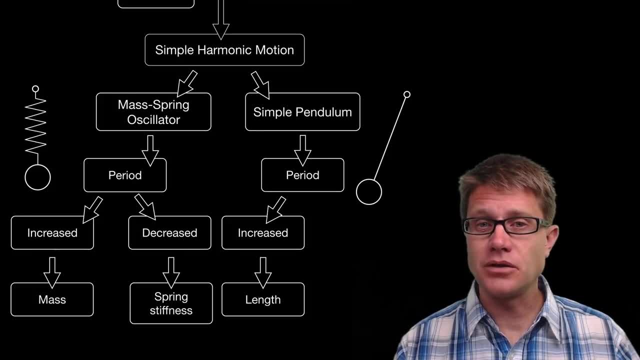 length of the pendulum. Now, what is interesting about pendulums is the mass does not have anything to do with it. And so how do we then decrease the period of the pendulum? Well, we have to change the gravitational field strength As we increase that field strength. 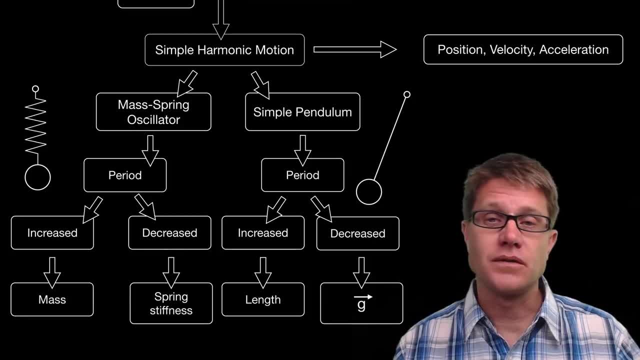 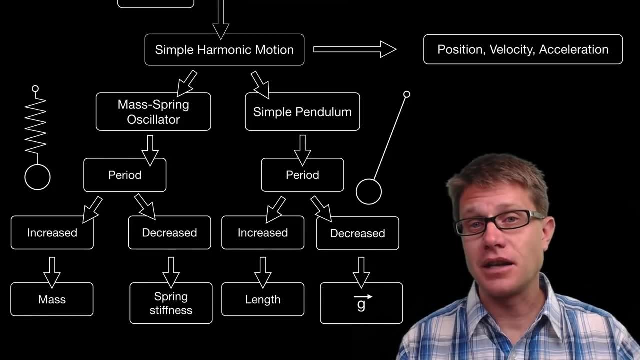 then we are going to decrease the period, And so, with both of these forms of simple harmonic motion, you should be able to identify the position of the object at any time, its relative velocity and acceleration, And figure out when these are at a maximum and when they are at a minimum. And so let's look at some 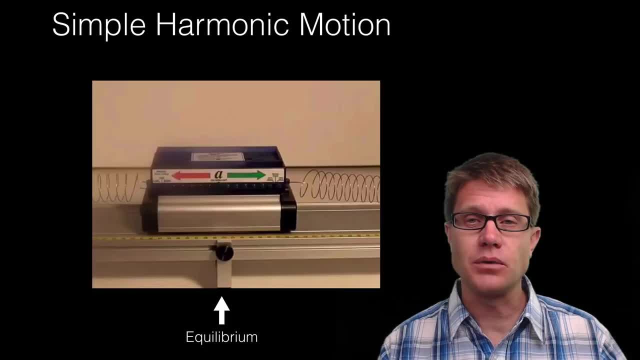 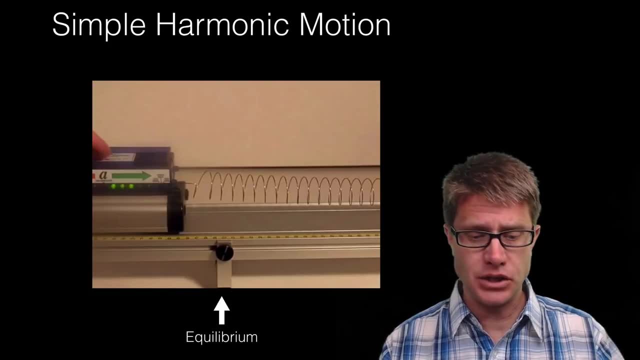 simple, harmonic motion. This one. we have got it horizontal with two springs, And so we can see its motion. Equilibrium is going to be right in the middle And so, as I pull it towards this side, there is going to be tension in this spring, right here, And it is going. 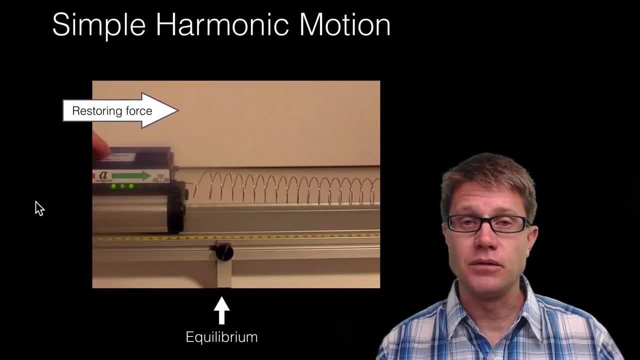 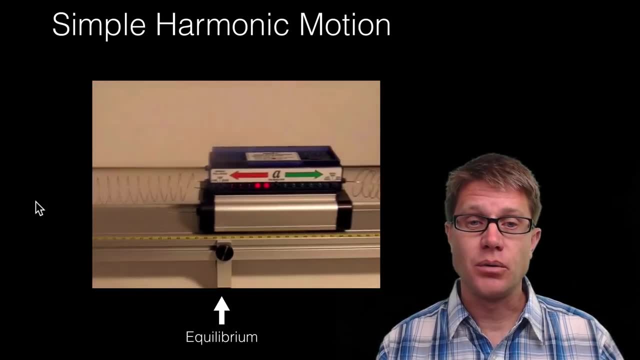 to pull it towards the right, And so that restoring force is going to move it towards equilibrium. Now it is going to move in that direction. Now this other spring is going to move it back towards equilibrium, like that, And so what we are going to get is this simple: 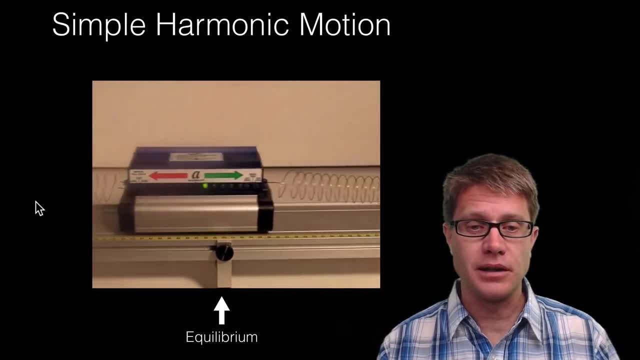 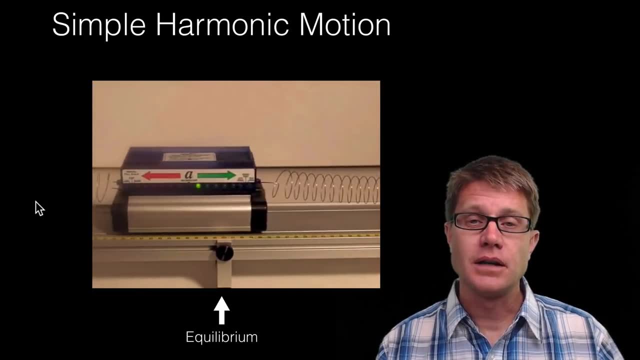 harmonic motion. What is cool about this one is there is an accelerometer with little LEDs so you can see the acceleration of the object. You can see right in the middle. there is no acceleration right in the middle, And so what do you have to do in videos like this or in 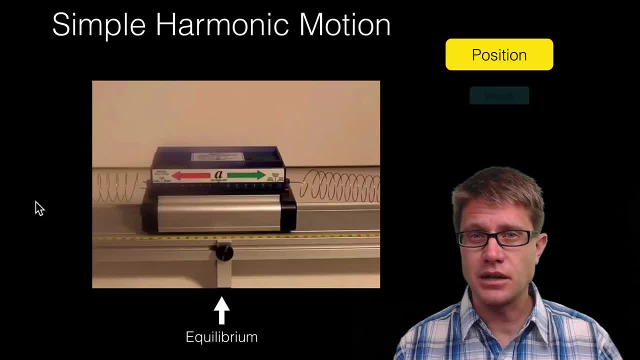 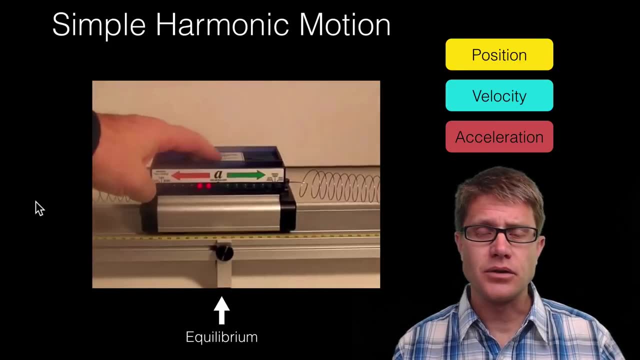 problems like this, You have to be able to identify the position of the object and the velocity and acceleration. When are they at a maximum, When are they going to be at a minimum? And so let's use this scenario. And so I am going to pull that object towards the left. And so now I have 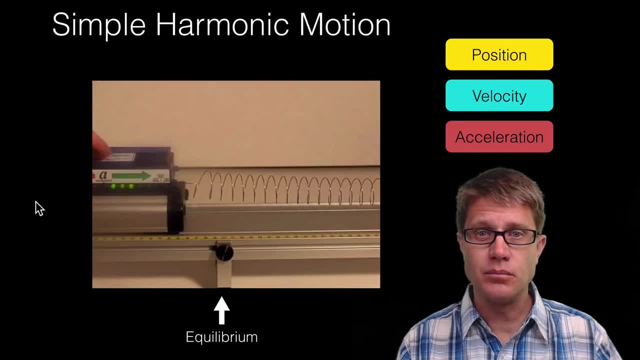 let it go. And so, at this point, right here, as it is starting to move, where is our position going to be? It is going to be maximum, towards the left. What about our velocity? at this point? It is going to be minimum, It is going to be 0.. And what is going to be our acceleration? 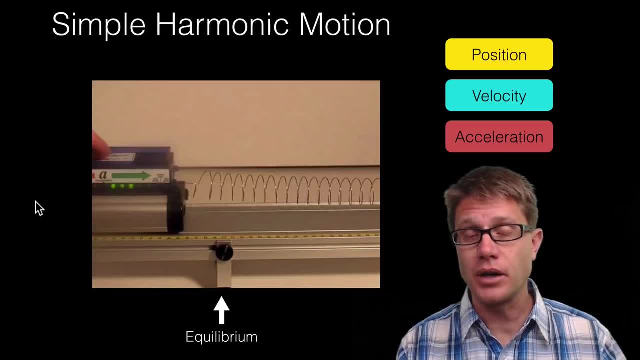 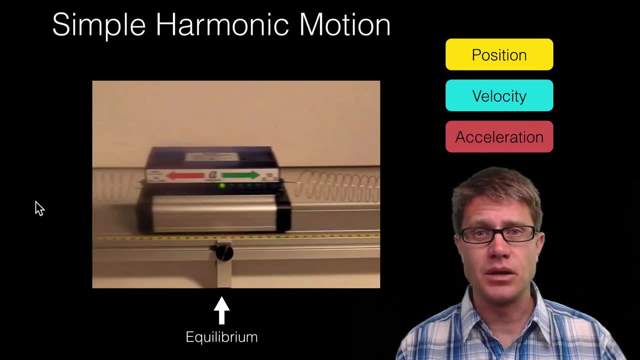 Our acceleration is going to be maximum towards the right. We are going to have great acceleration at this point. Let's let it go for a second, And I have paused it again here, right in the middle. What is our position? Again, it is minimum, It is at 0.. What is our velocity? Well, it is accelerated. 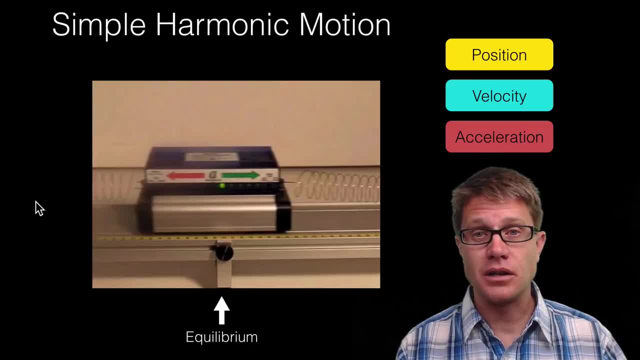 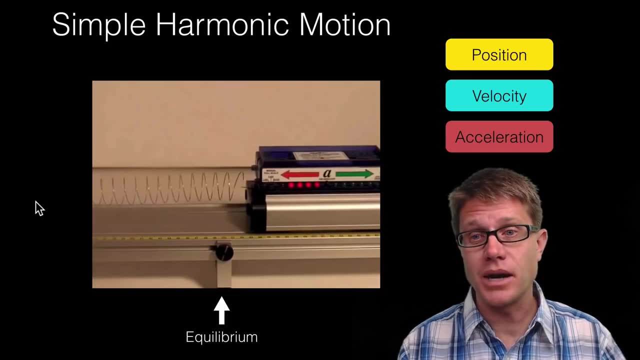 and now our velocity is at a maximum. at this point. What is our acceleration? There is no acceleration, right when it is in the middle. Let's let it go again. It is going to move over to this side. Now our position is maximum to the right. What about velocity? It is back. 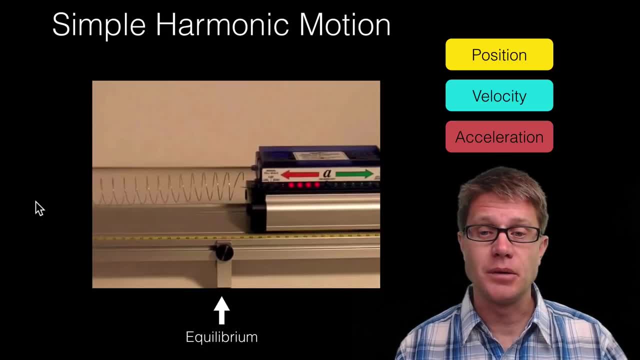 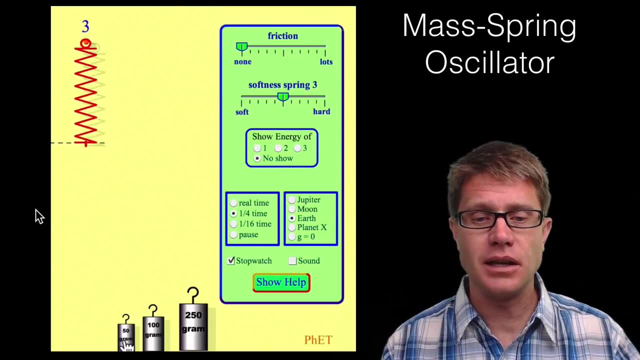 to 0 again. Where is our acceleration? It is going to be maximum now towards the left, And so let's do some little experimentation with the mass spring oscillator. We are using a PHET simulation And let's look at how the mass and that stiffness of the spring 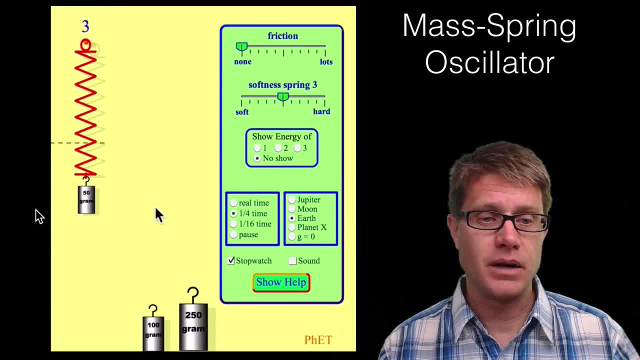 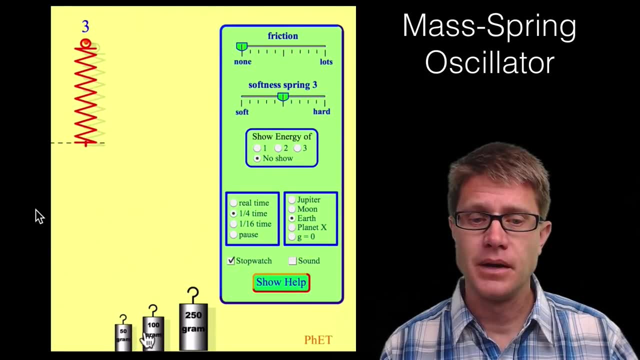 affect the period, And so I am going to take a weight and put it on here And then we will measure the period just qualitatively. So that is going to be the period. So that is a 50 gram mass. Now let's put a 100 gram mass on there And let's listen to the period. 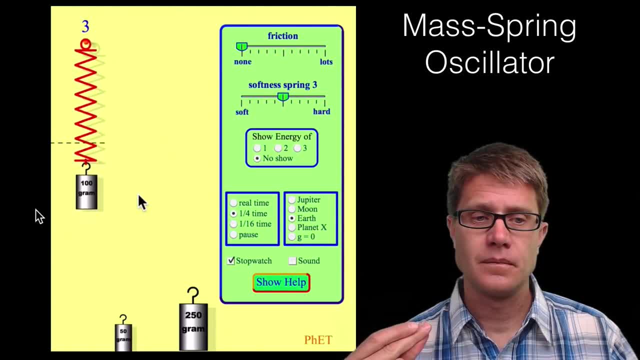 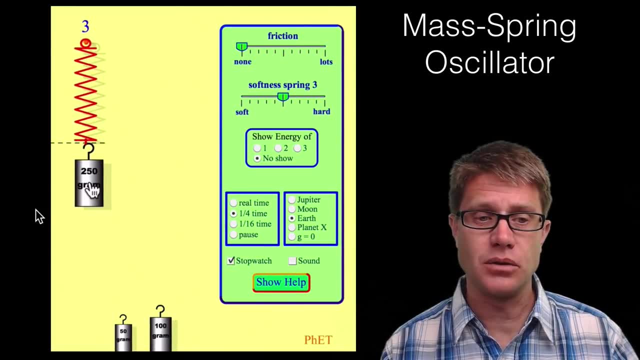 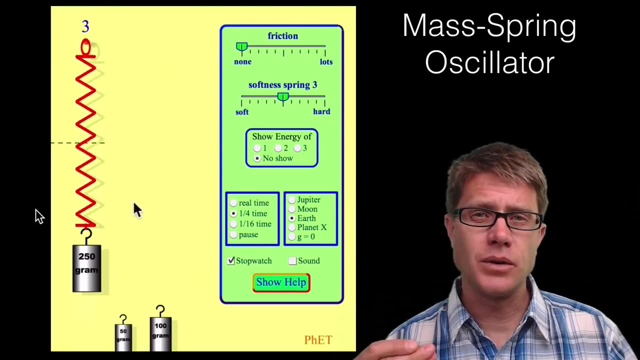 again. Okay, So you can see that we are slowing down the period as we increase the mass. Let's put a 50 grams on there So you can see that as we increase the mass on that spring, then we are increasing the period. But now let's play around with the stiffness of the spring. 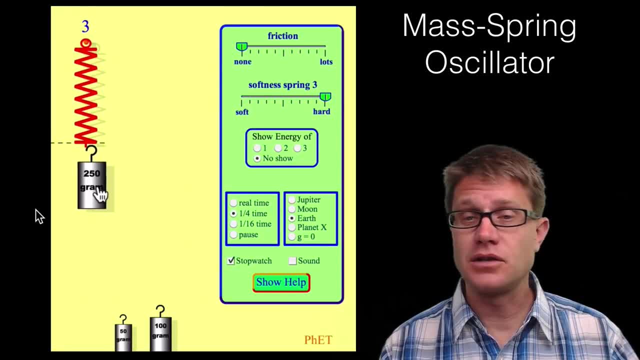 We call that the spring constant. So now I have made it a stiffer spring, I put that 250 gram mass on it And you can see the period is now decreasing. And so by increasing the stiffness of the spring, we are increasing or decreasing the period, rather of the spring. 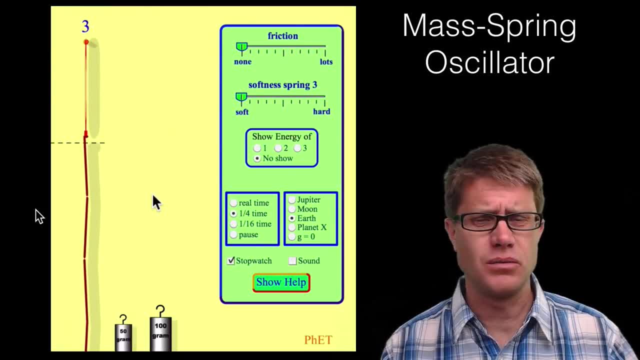 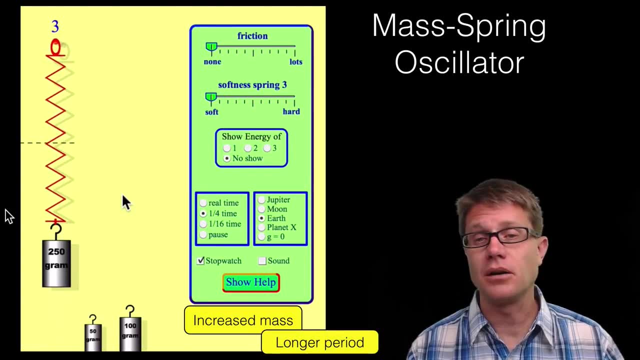 Now let's really make it a soft spring. What happens, You can see the period gets really, really large. And so, in summary, what have we learned just from this experimentation? that if you increase mass, you are going to be make a longer period For that harmonic. 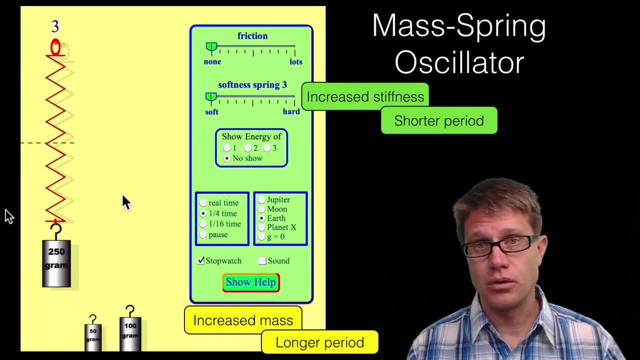 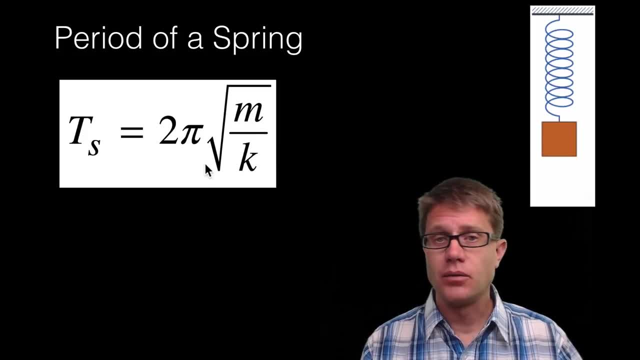 motion And if we increase the stiffness, then we are going to make it a shorter period, If we look at that quantitatively. so if we look at the actual period of a spring like this, what is really affecting it are two things: The mass and the spring constant. 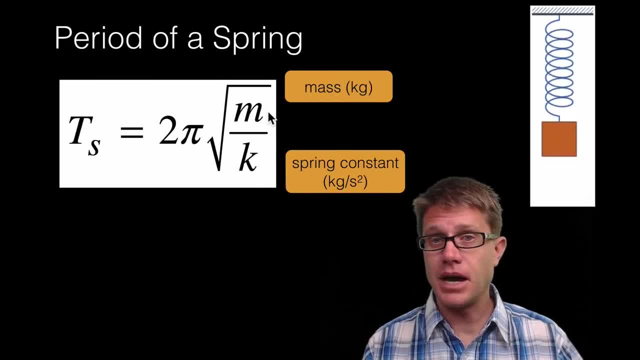 And so you can imagine, just looking at this algebraically, if we increase mass, what is going to happen to the period? The period is going to increase because it is in the numerator. What is going to happen if we increase the constant of the spring, or the spring constant as we make it stiffer? 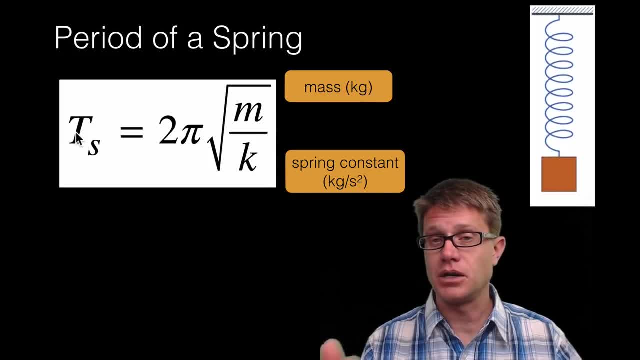 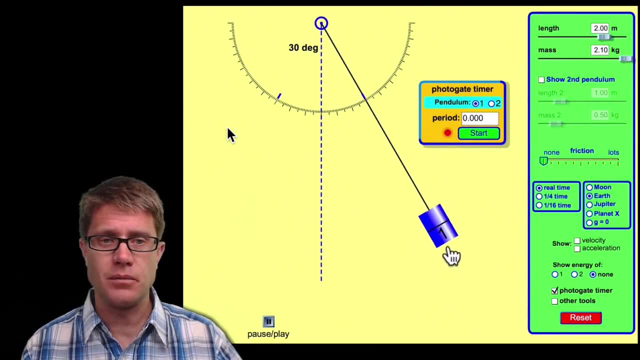 as this number gets larger in the denominator, Then we see that the period is going to become less. Now let's look at a pendulum- Again another PHET simulation. So I am going to move this to the side, I am going to try to drop it at about a 30 degree angle And this: 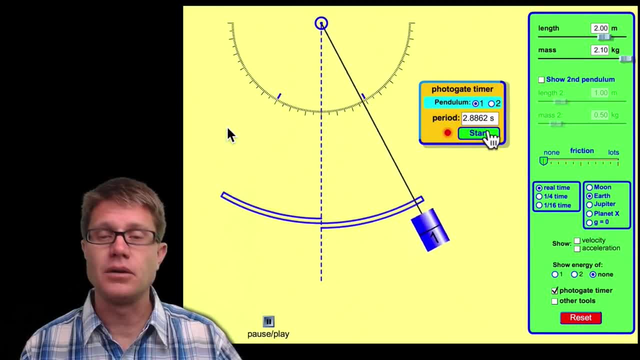 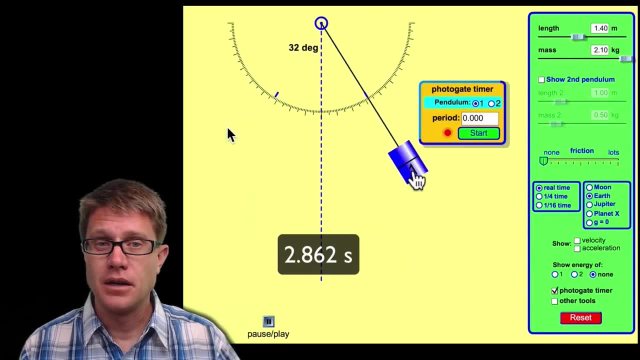 one has a little photogate timer so I can time how long it takes to get back Or how long it takes to get back to that original position. So we can see here that we have got a period of 2.862.. Now I am going to make the pendulum have a smaller length dropping. 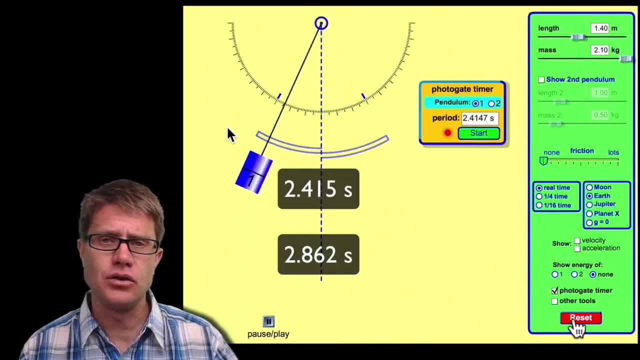 it from the same angle And you can see that the period now is less. It is 2.415.. Now let me make it even less. I am going to try to drop that weight again at a 30 degree angle. Set my photogate timer And you can see that the period is becoming less, So as we decrease. 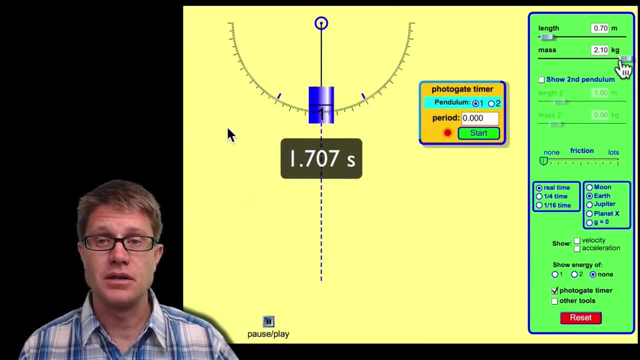 the length. what are we doing to it? We are speeding it up or the period is decreasing. Now watch what happens as I change the mass. now, As I change the mass, drop it from a 30 degree angle. start my photogate timer. you can see that it does not affect it. So 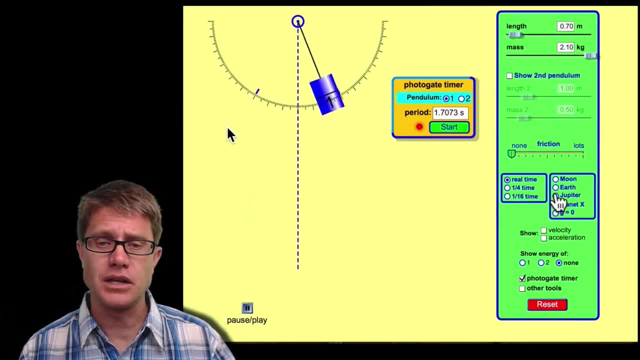 mass does not affect the period, But what does remember is going to be the gravitational field strength. So now let me change it to the moon And you can see that the period is increasing. It is slowing down. Let me change it to earth Now: it is speeding up. 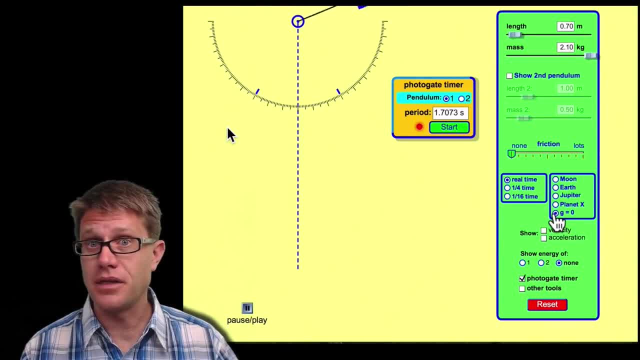 What happens? if we make it Jupiter, It is really speeding up, Or if we make it nothing, It just continues moving like that. Now we are moving over to the moon. Let's get breathe. So, as you can see, here we are shifting the period, And now we can see the time Again also.